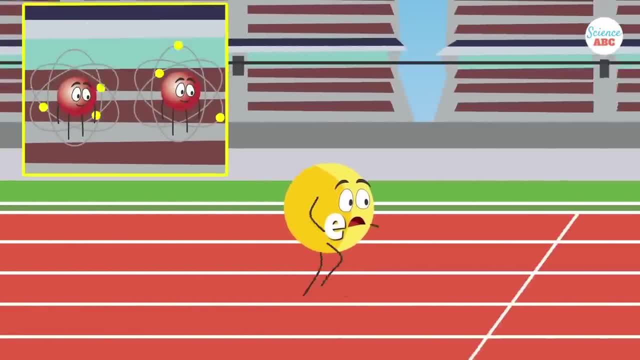 you may incorrectly assume that you can estimate its position in the next few moments. However, if you measure the position of a particle, say an electron, as it moves along its trajectory, you may incorrectly assume that you can estimate its position in the next few moments. 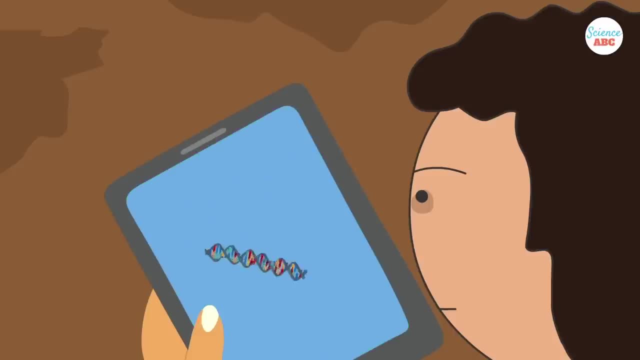 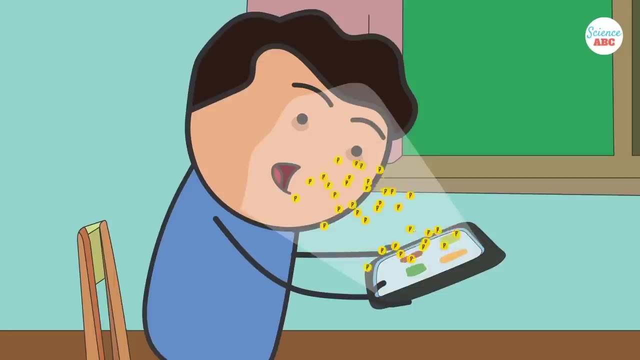 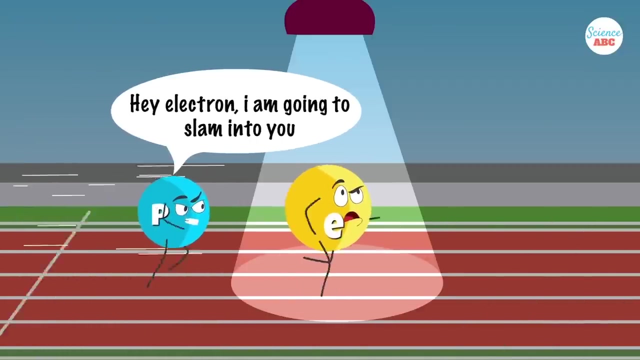 Consider this: You were able to watch this video because packets of light, called photons, bounce off your screen and reach your eyes. Those photons of light are what enable you to see this video. On the contrary, seeing something as tiny as an electron is not so straightforward, If you. 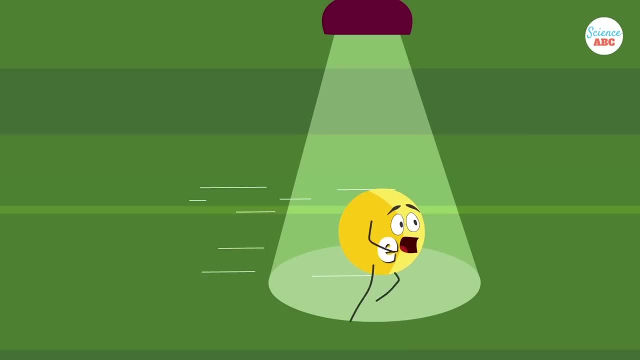 bounce a photon off it and try to detect that photon through an instrument, it's likely that the photon will impart some amount of energy to the object. If you bounce a photon off it and try to detect that photon through an instrument, it's likely that the photon will impart some amount of energy to the object. 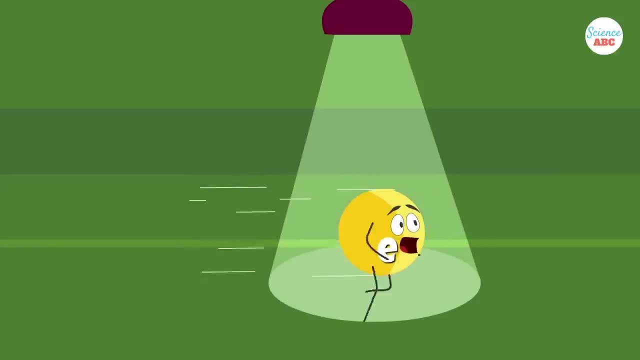 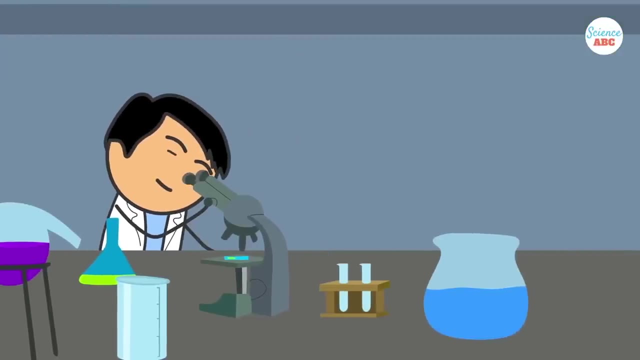 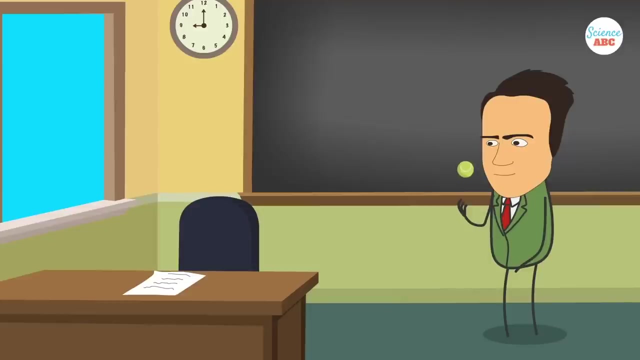 As a result, the electron's path will no longer be the same as it was earlier. This is why your observation of either the position or the momentum of the electron will be inaccurate. This is the idea upon which the Heisenberg Uncertainty Principle is based. Werner Karl Heisenberg. 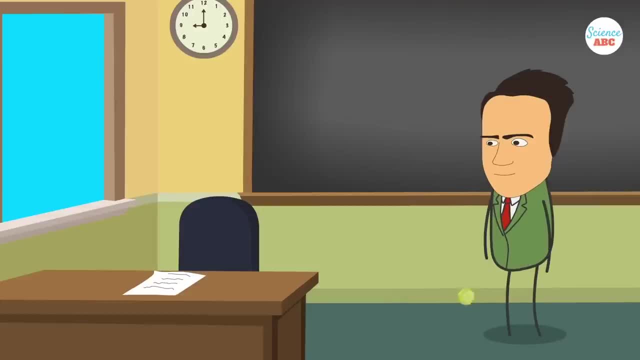 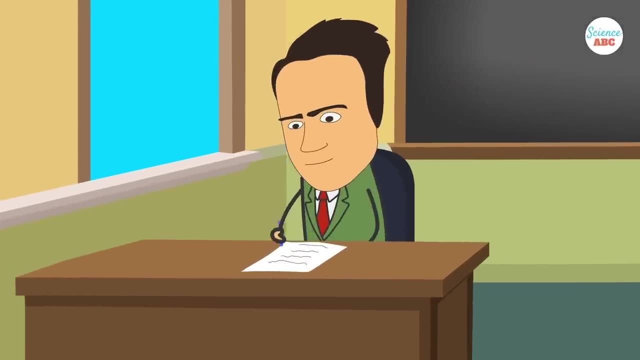